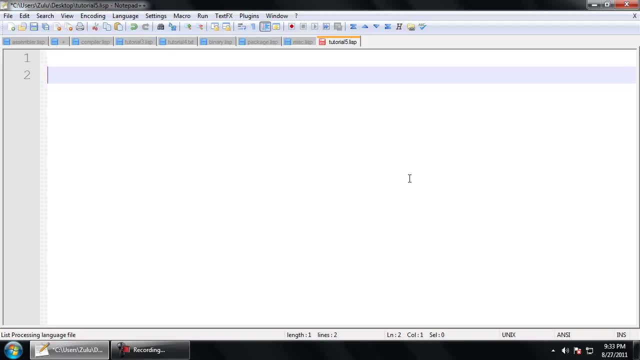 just call it something else I'm going to do, as my professor used to do, and just add an m in front of it. That stands for my length of a list. So very similar. If we have a null list, the length is: 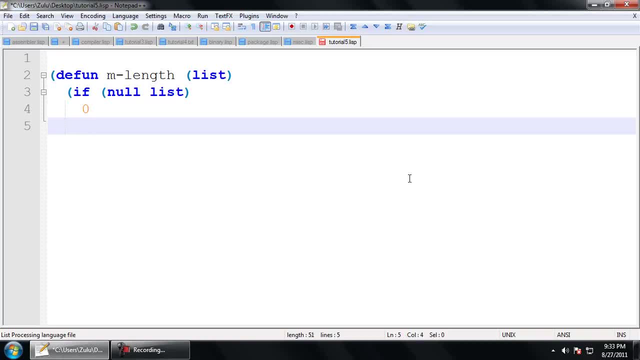 by alternate qualities: zero. But if instead we have at least one element, then we can go ahead and just add one Right, Just the the, because we can definitely count one element, but we can't say anything about the rest of the Lisp. 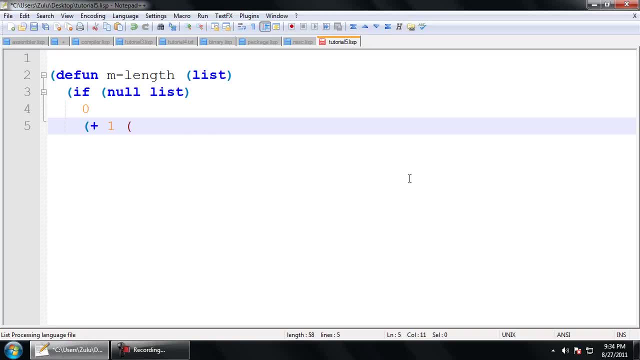 So what we're going to do- go ahead and do- is add one and then take the length of the rest of the list, Which is by using cooter. Alternatively, what you could have done was just define a. you could have done this. 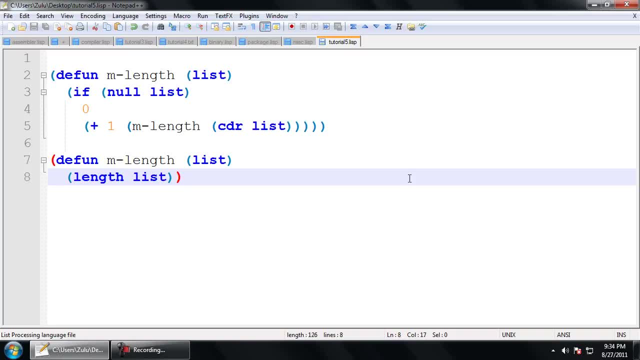 And probably a bit more efficient solution as well, But nonetheless I'm trying to show you know, getting you comfortable with recursive relations like these. Alright, other quick function: printList. to print a list And we have nothing to print in this case. 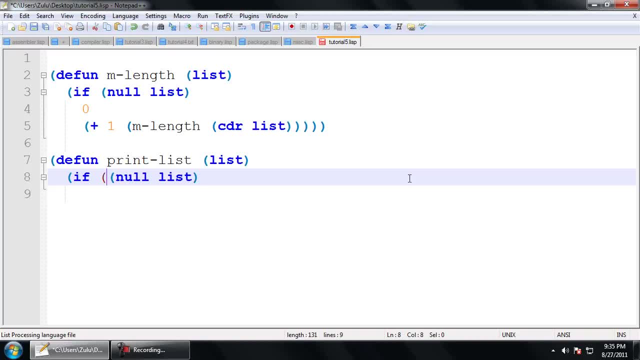 So what we're going to do is not So if the list is not null, By alternatives, you could have just put if list, because if list were null, it would be nil, In which case this would not be true. So it's the same thing, but just because we're trying to. but when you use it this way, you're. 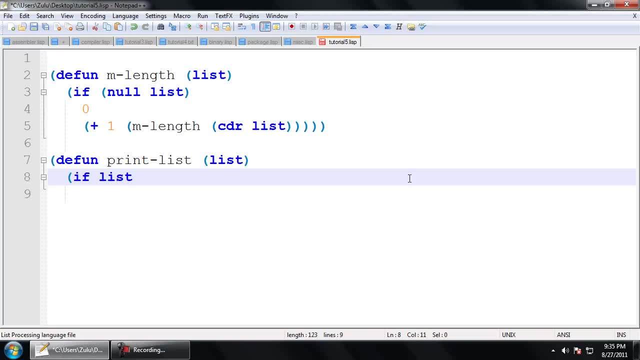 you're? You're. You're trying to use list as a Boolean value And while it's right in terms of data types, it's wrong in terms of syntactically, when you're thinking about the program. In most cases, I would be fine in just writing this. 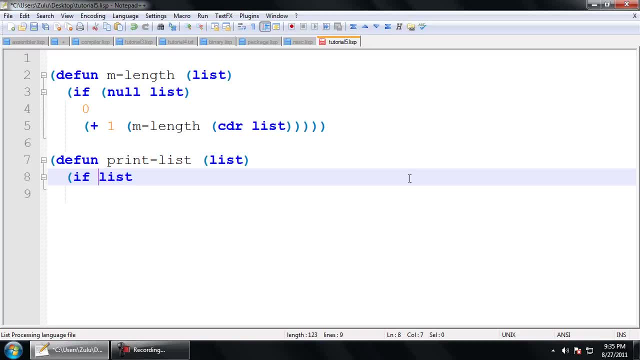 But here just to emphasize that we're using nil as an empty list. what I'm going to do is take this approach instead. So if it's not null, then what we're going to go ahead and do is just print the current element. 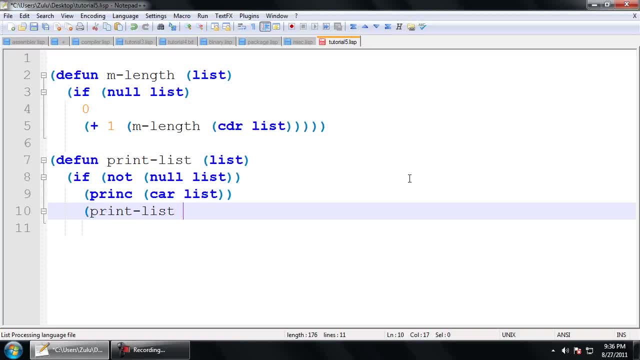 And then we want to go ahead and print list on the rest of the elements, right, But oh no, If we put this here, what it's going to be is: this is going to be the else expression. So what we're going to use here is a. 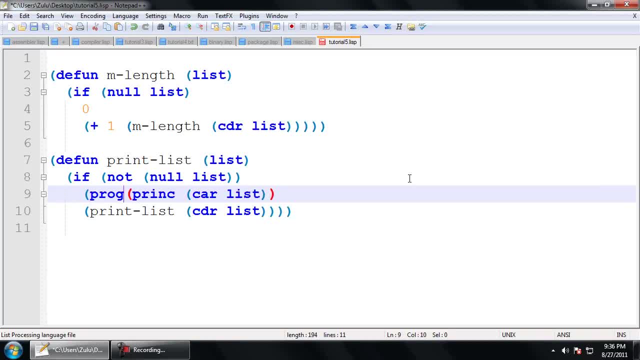 Here is a new special operator, which is prog n. Prog n is essentially opening up a block, you know, like the curly braces in C. The other approach is to use let and then give it no arguments, you know, no variables. 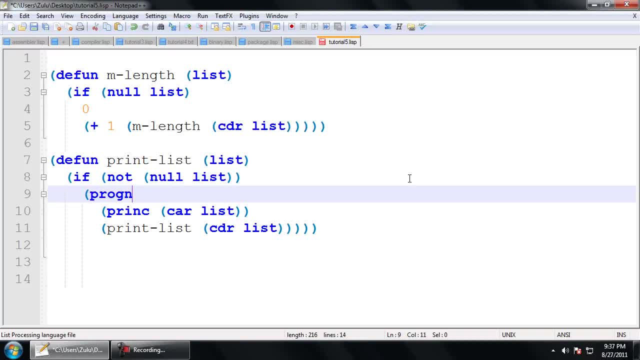 But prog n is much better in this case because we don't need any variables. So why use let All right, So that'll take care of that. because this entire thing is considered the consequent. So that'll only happen when this is true. 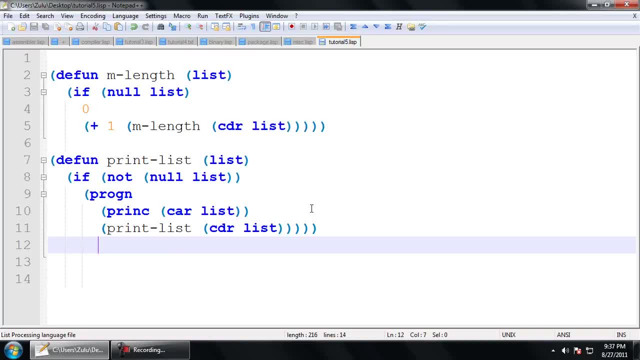 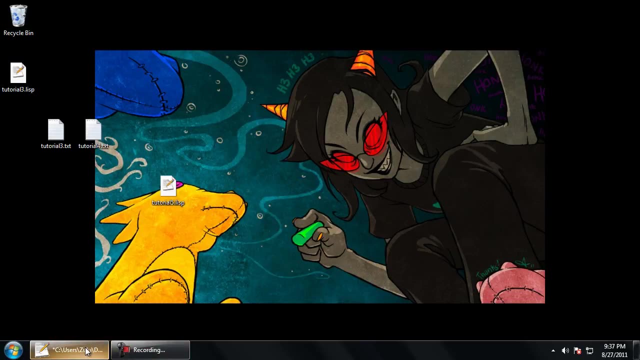 All right, Let's see another one. So how about we revise that sum function we had from before? Let's go ahead and get that from. All right, Let's see. Since I renamed it, it actually deleted the old one. Oh well. 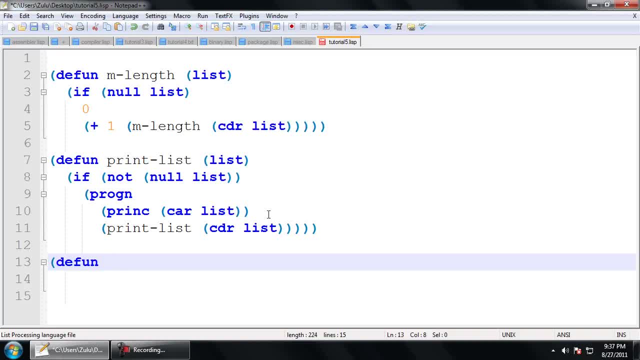 Defund sum right, So let's call it sum numbers. So in this case we cannot assume that the list contains only numbers It may contain. So in this case it may contain either numbers, it can contain symbols or it'll contain lists. 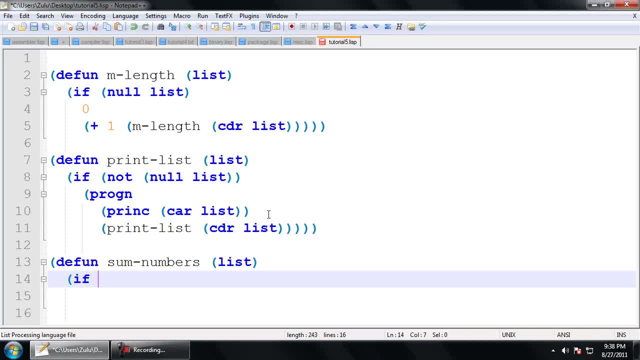 So what we're going to want to do with this function- this is going to be considerably more difficult- kind of- is: we want to go through any list and we want to find every single number in it, So we could have a crazy list such as you know. 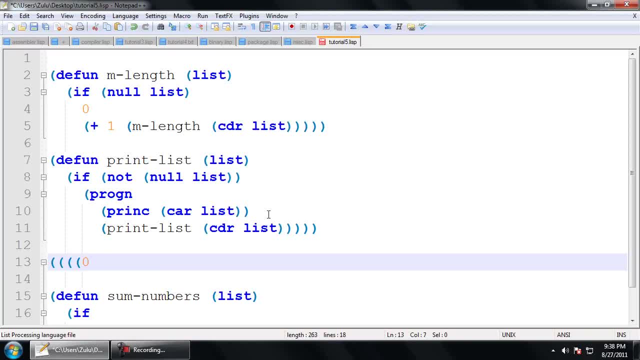 A bunch of lists and 0,, 5, X, Then we have O, 1,, then A, Then we can have 0,, 1,, 0,, 2,, 3.. We can have a list like this, where the first element is this list, right here. 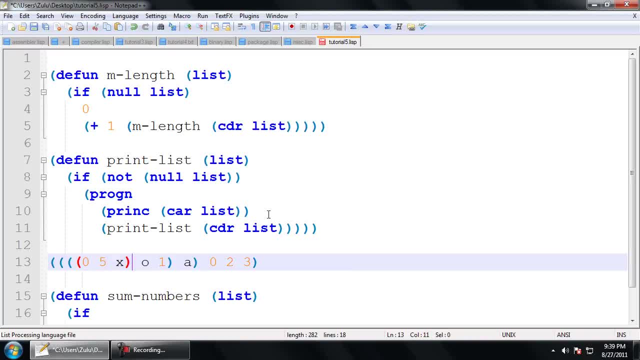 And the second one is 0. And this, So what we're going to want to do is grab this 0, let's make it a 1, so it's important. Let's make this a 7.. So, grab this 1, add it to the 5, add it to the 1, add it to the 7, add it to the 2, add. 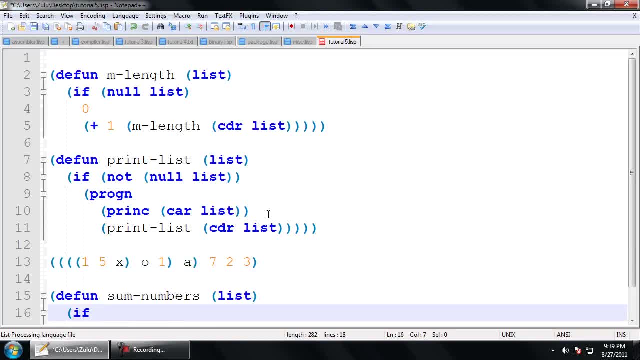 it to the 3.. So, since this is a bit complicated, we're going to have a lot of if-elses. I'm going to show you a quick macro called cond, And it's essentially like an if statement, An if. 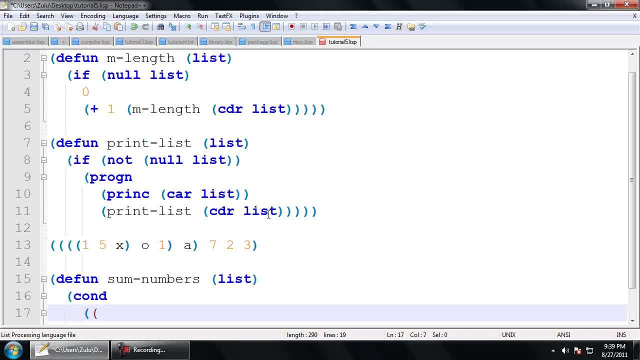 You know an if operator. However, what it's going to do is it's going to accept multiple conditions and then multiple consequence. So this is how we would write, say, if we were just doing the normal sum. We would write it as if null list here. 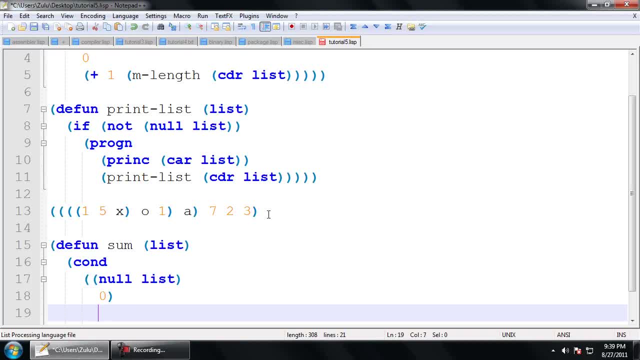 Then what we want to do is 0, return 0. So notice that We have a list. that is the condition And then the return. So, similarly, we're going to have a condition here And in this case, since, in order to do an else in a cond, what you do is type t. 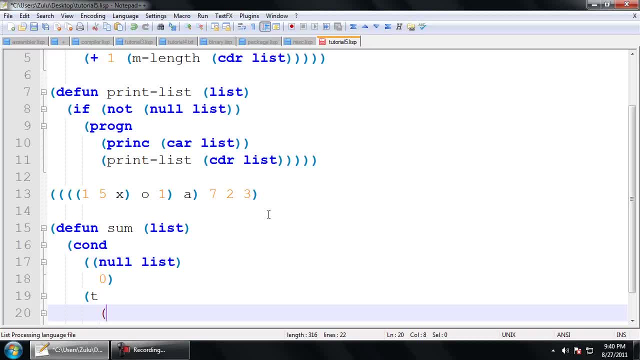 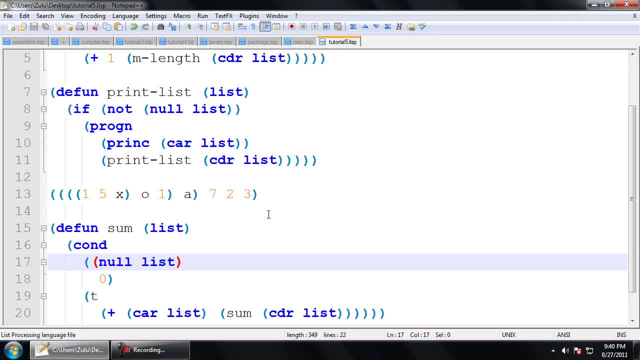 0. 0. 0.. So you'd see that this one we're going to write and see that this one is a hints list, And then we're going to write a list as well. So I'm going to drop a little it up. 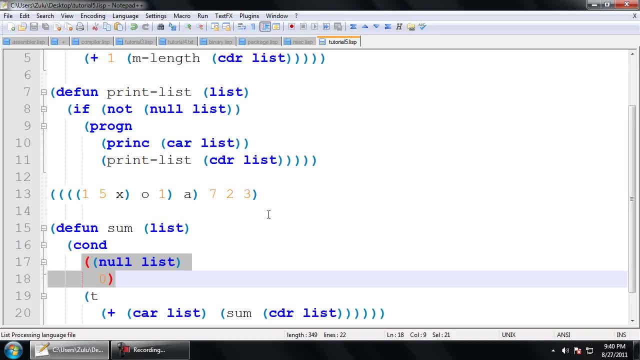 And it shows up in here, which will be our list of? not at all, but we'll just say a list. So we'll say a list of pairs And then we'll go back to it And then we'll see it. 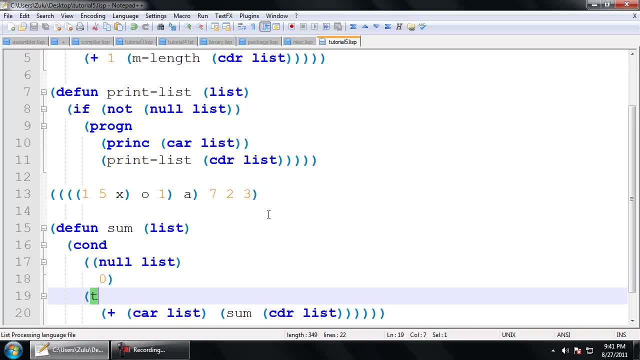 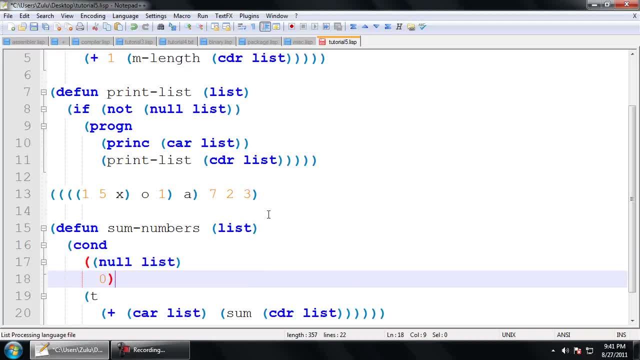 return 0. now, if we actually do have something in the list, that doesn't mean that that's something is a number. so what we're going to go ahead and do is we're going to say if what we have in the list currently, so the current element of the list, not EQ number P. this stands for number predicate. 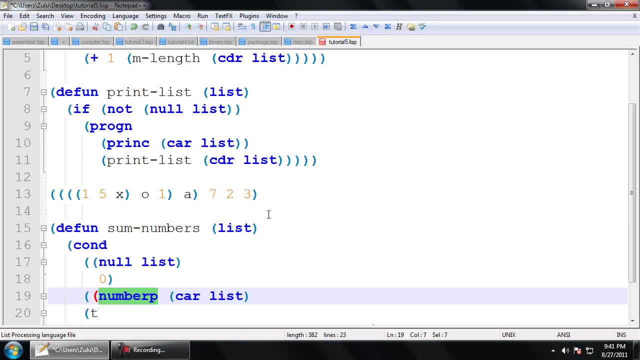 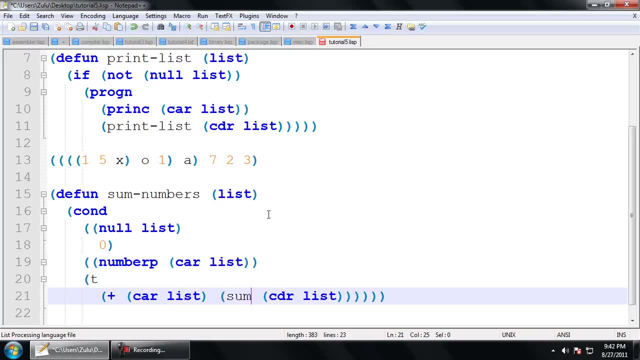 it's going to return 0, true. if it's a number, false, otherwise. so this is exactly what we want. so if it's a number, this is actually what we want to do, right, then we can say: if it's instead a symbol, so if symbol P, then we. 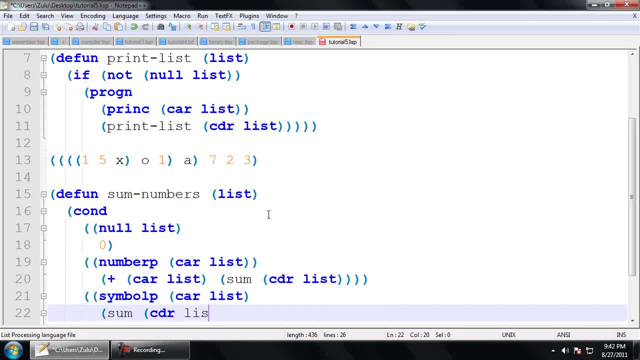 just want to return the sum of the rest of it. now, if it, what if it was not a number and if it's not symbol? what I said was that it's either it's either a number, it's a symbol, or it's a list. so what we can do, 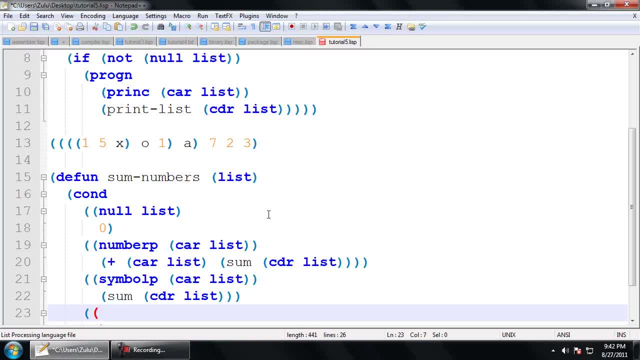 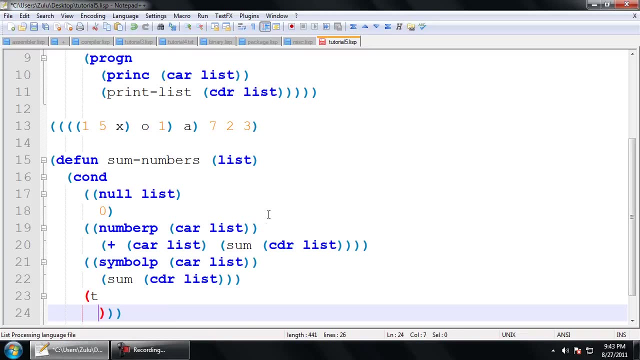 here is. we can either say: you know, test it for it being a list by using list P. however, since we know that that's the only other case as far as what I specified it to be, we can use use T as a as an. else, and similarly to what I do and see, I would write something like this: 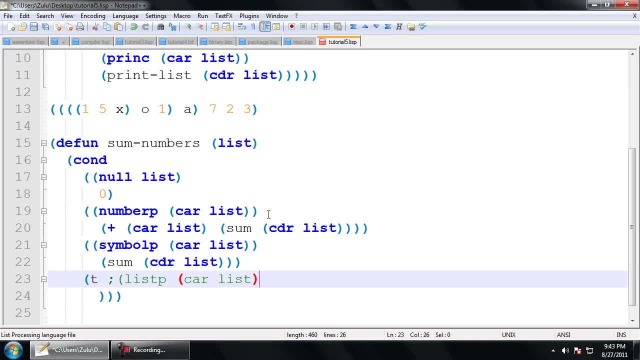 just to say what that stands for. all right, so in this case, what we want to do is we want to add the sum of that, that sub list, with the sum of the rest of the list, and this it's very- I think it's very important for you to understand this example, because if you can understand this, you can do many. 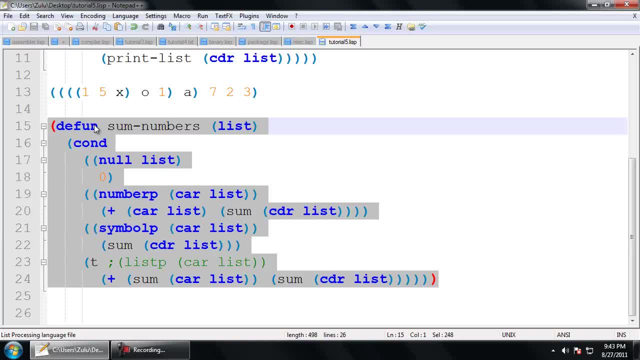 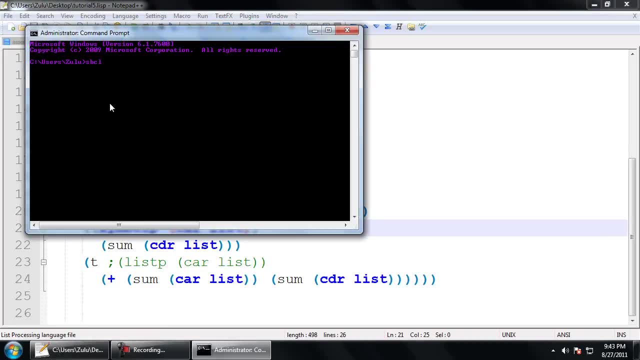 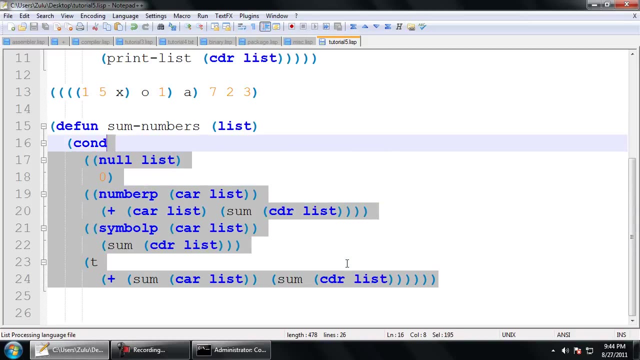 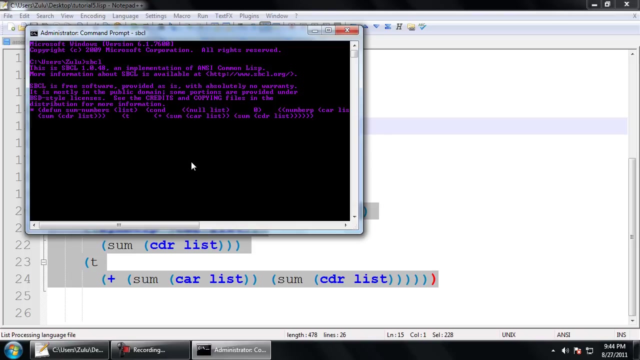 other list operations, no matter how complicated though the list is. so let's go ahead and toss that into the REPL so you know you can get a little more assurance that it does work. and the reason I deleted that comment was that for some reason, when I copy paste here and there's a comment present, that is: 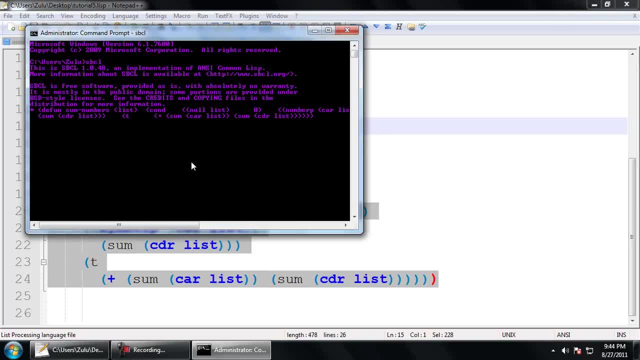 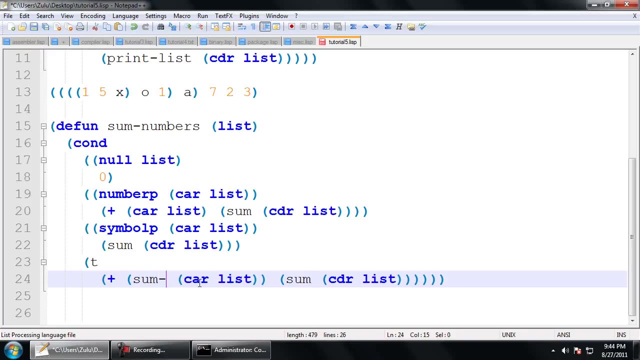 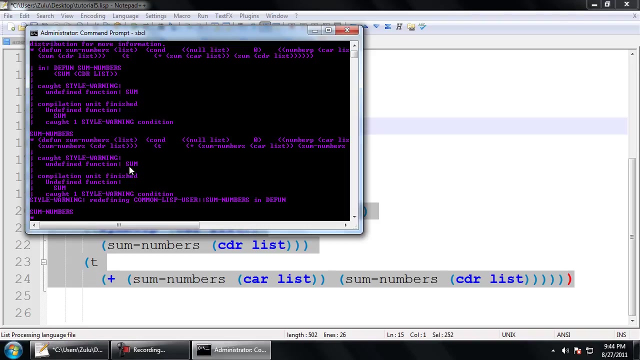 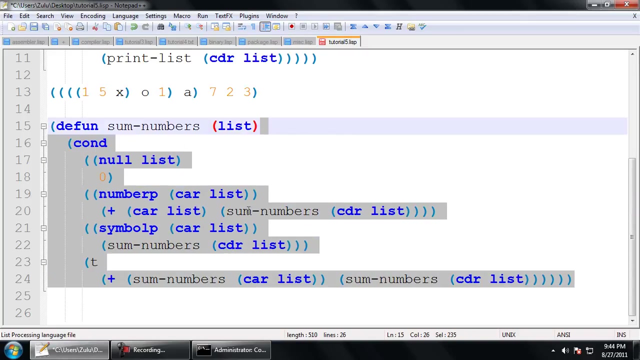 specifically on Windows, when there's a comment present, it will take up some of the like the other forms, so just make sure that. okay. what's happening here is that we don't have a function called sum. it's some numbers, all right, let's grab that. I'm sorry about that. all right, just install a warning saying that we're. 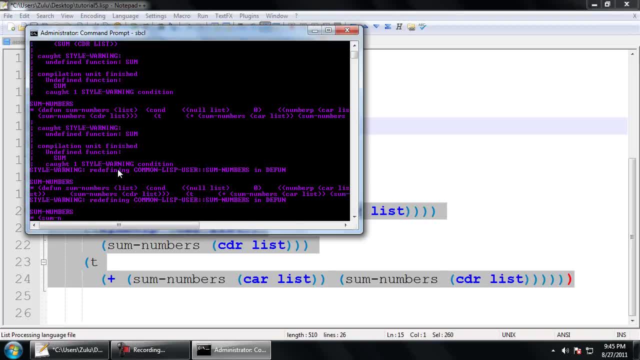 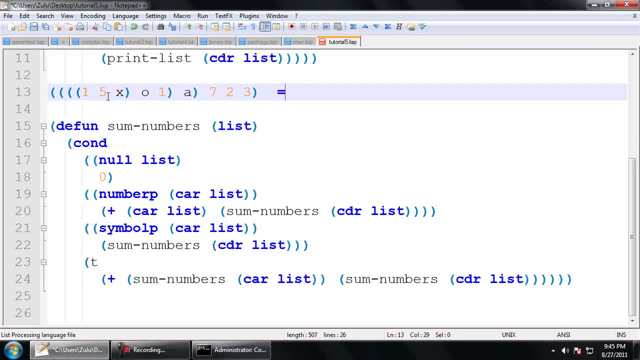 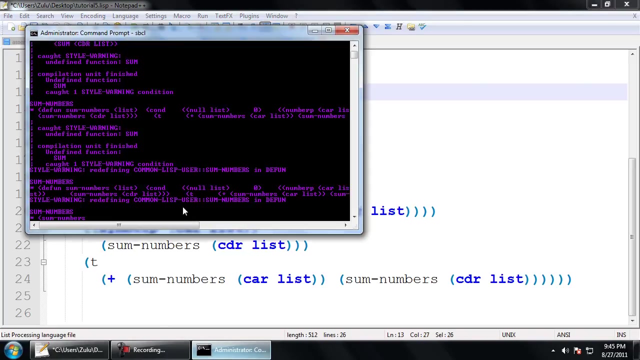 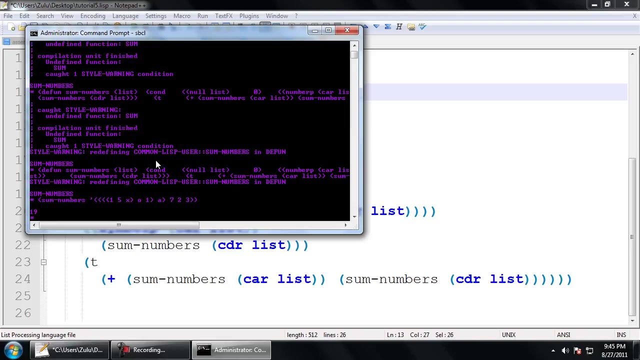 redefining it. all right, so if we have some numbers, so let's give it that list that we had here. the result of this should be six, seven, fourteen, sixteen and then nineteen. let's go ahead and quote that so you can copy and paste it. and there we go: 19 now when you're testing out some code, a very useful